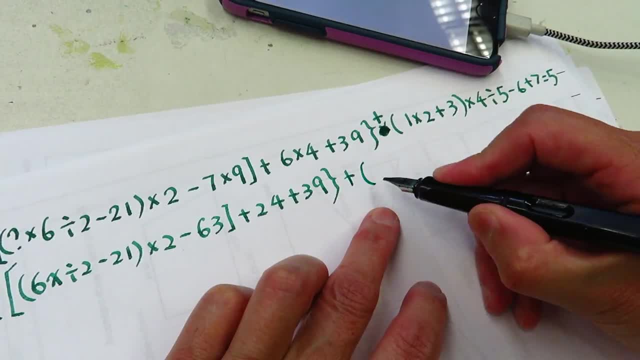 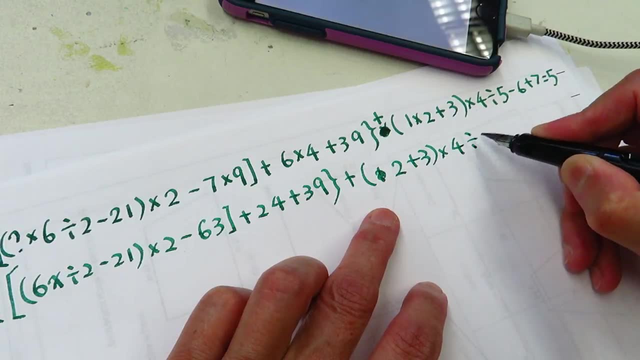 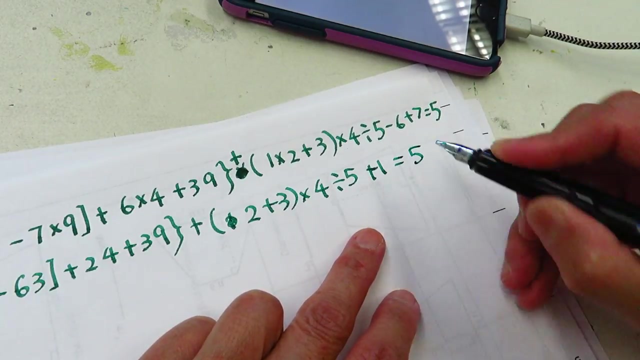 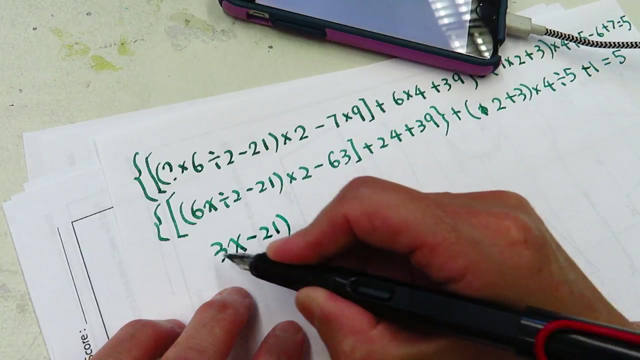 Let me try to make it 1 times 2 plus 3 times 4 times 5 minus 6 plus 7 plus 1 plus 5 plus 7.. So 3x minus 21 times 2 minus 63.. 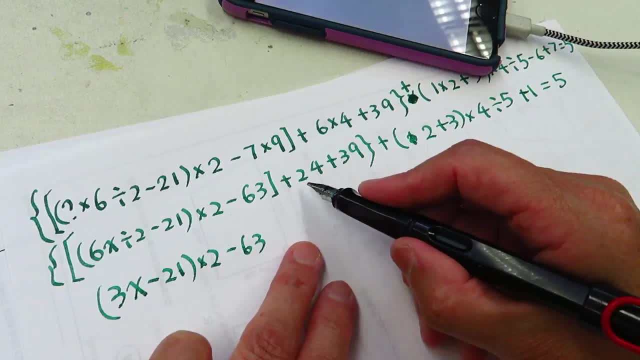 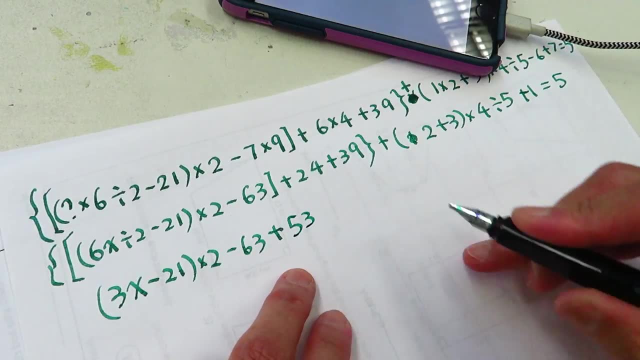 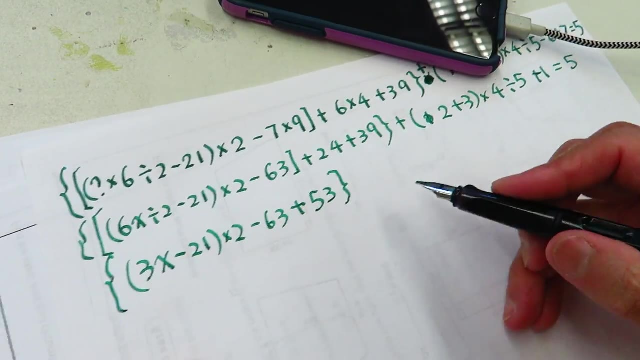 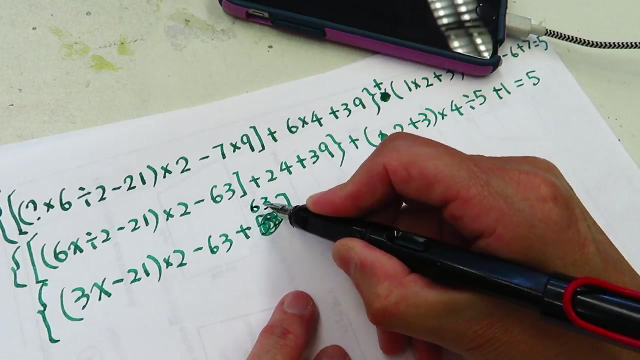 Right, This one: 24 plus 39 plus 53.. Right Plus 53.. 24 plus What I'm thinking, 24 plus 39. 63.. I was looking at the mirror And 2 plus 3 equals 5.. 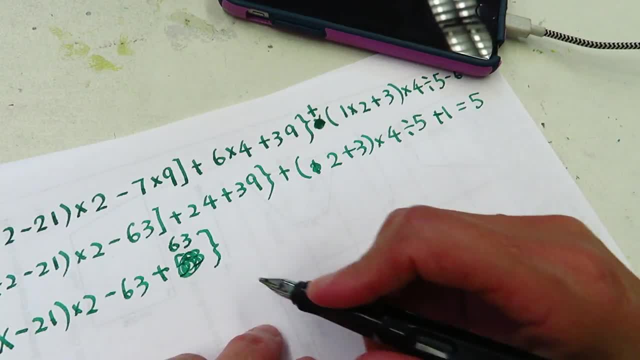 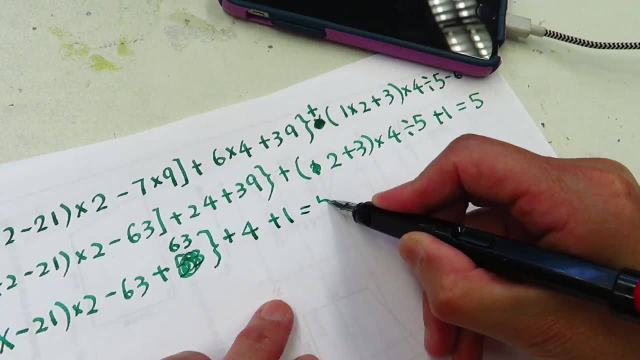 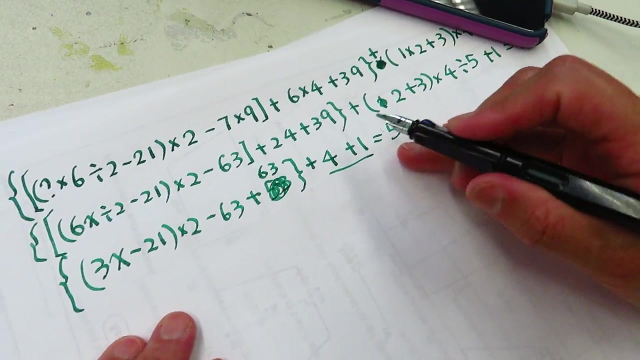 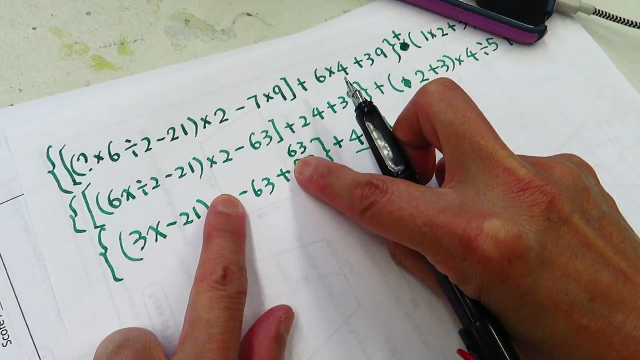 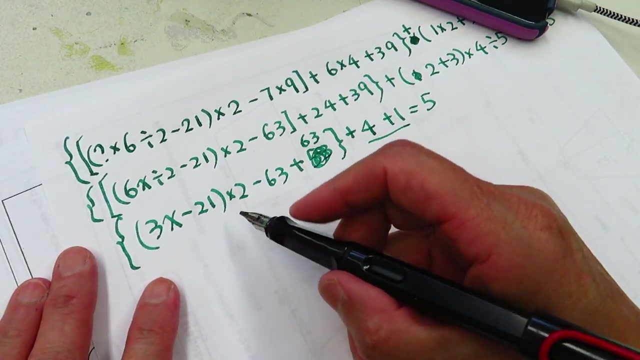 It becomes clear. So this positive 5, positive 5, we can get rid of, And it means this side equal to this side. Negative 63, positive 63, it's 0. So this becomes 0. And 2 plus 3 equals 6.. 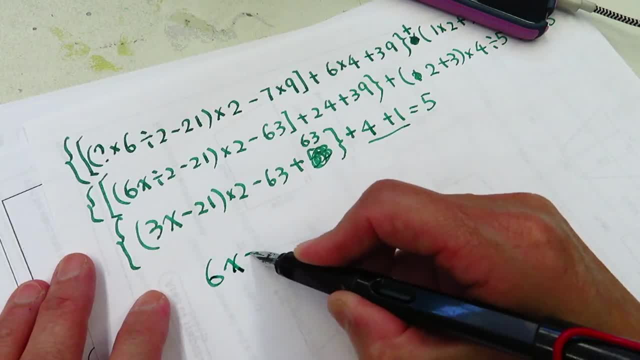 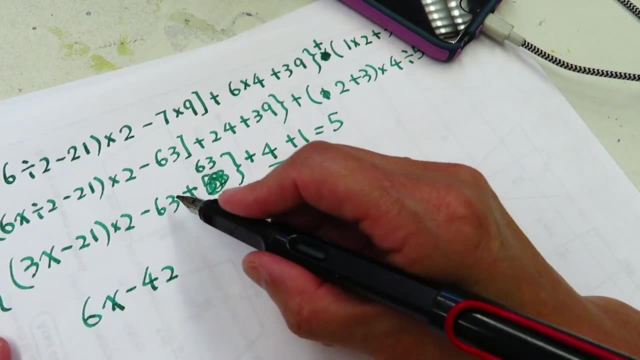 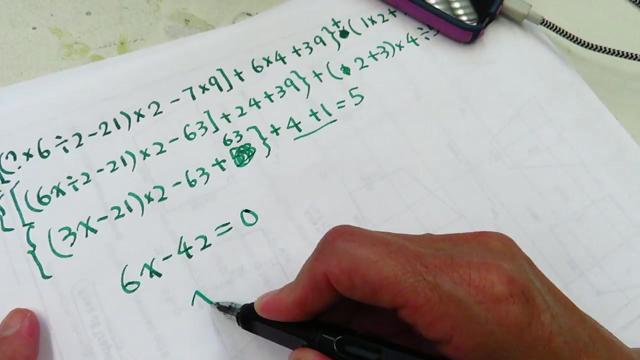 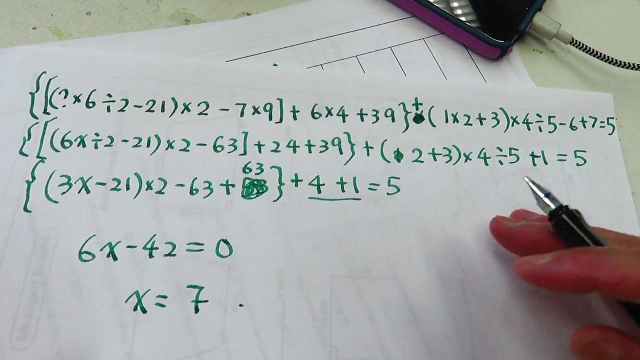 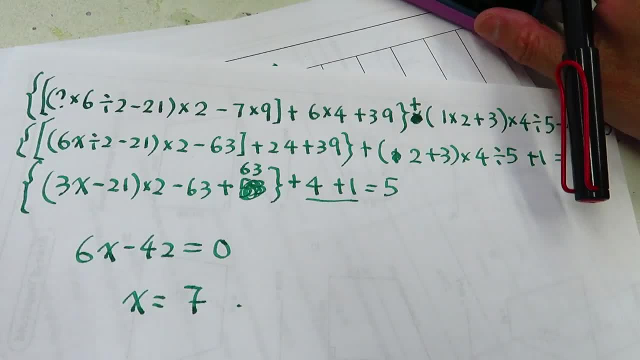 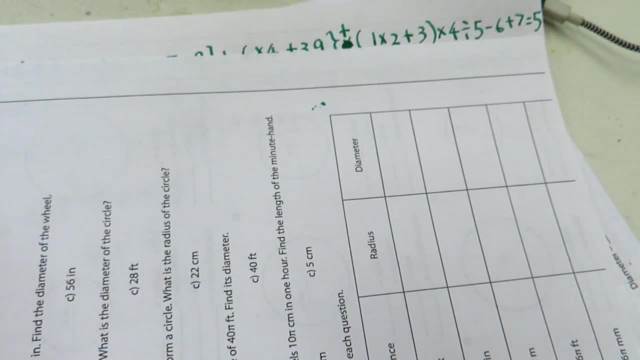 It takes him some time to work out, But when you see it it's really fun to see the problem. But when you see it it's really fun to see the problem. Here is another student trying to make some problem. I like 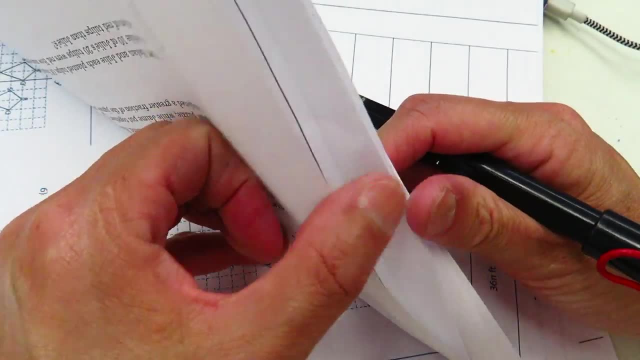 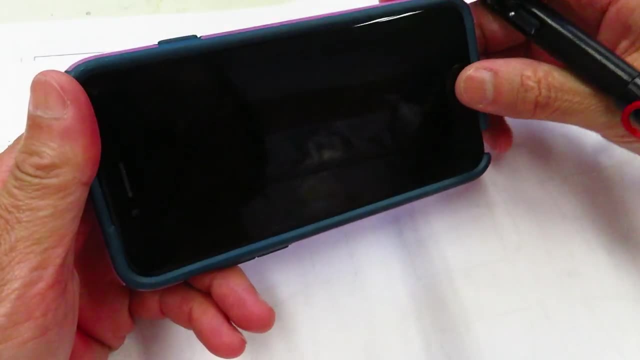 They are playing with numbers. They are playing with numbers. Let me see if I have any sketch here. Let me see if I have any sketch here. Okay, We will look at this. I have calculated and the result is not that. I have calculated and the result is not that. 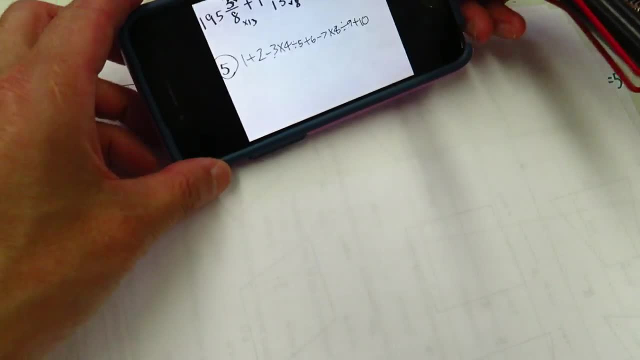 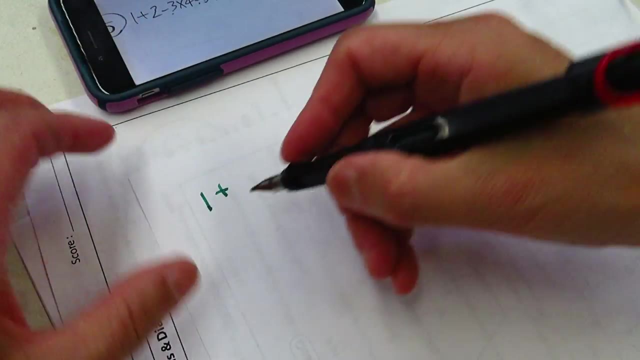 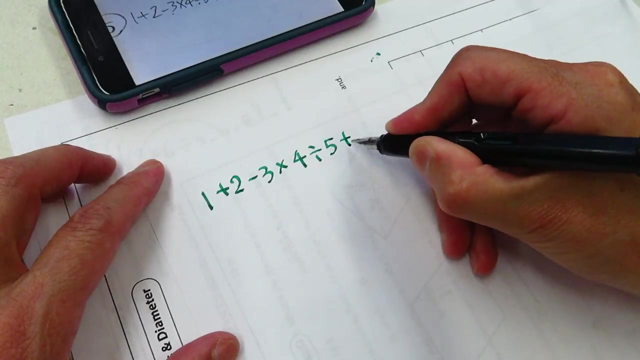 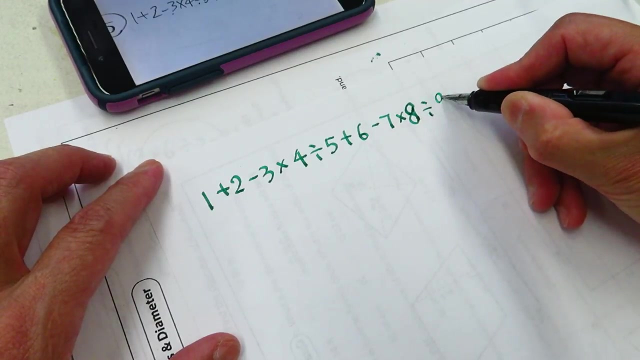 I have calculated and the result is not that That's even, But let's do it: 1 plus 2 minus 3 times 4 times 5 plus 6 minus 7 times 8 times 9 times 10.. The result is not. 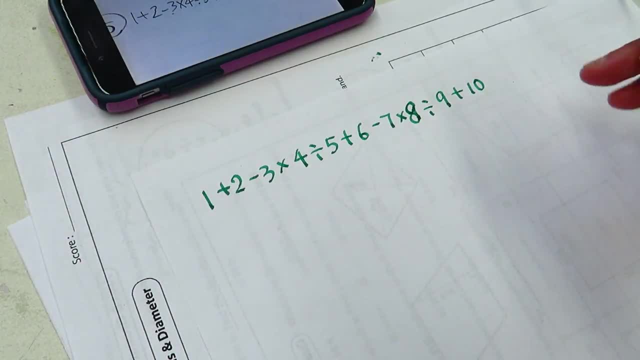 It's 1,, 2,, 3,, 4,, 5,, 6,, 7,, 8,, 9, 10.. It's 1,, 2,, 3,, 4,, 5,, 6,, 7,, 8,, 9, 10.. 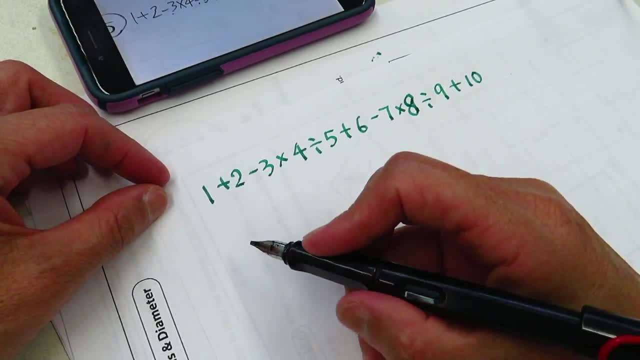 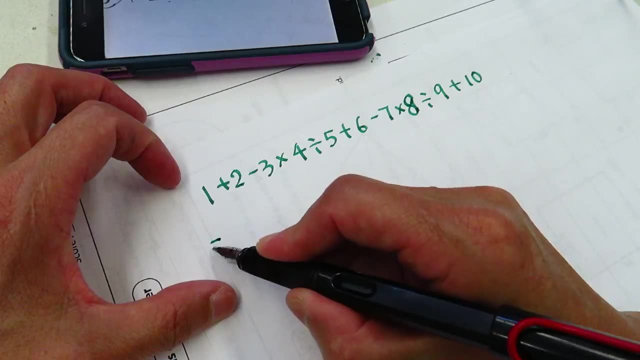 From 1 to 10.. But this number is not special. This addition and subtraction is used very well. This addition and subtraction is used very well, But this number is definitely an incomplete number. Let's calculate together: 1 plus 2 can be divided. 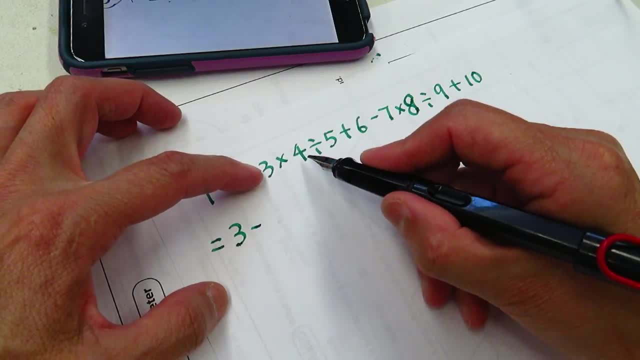 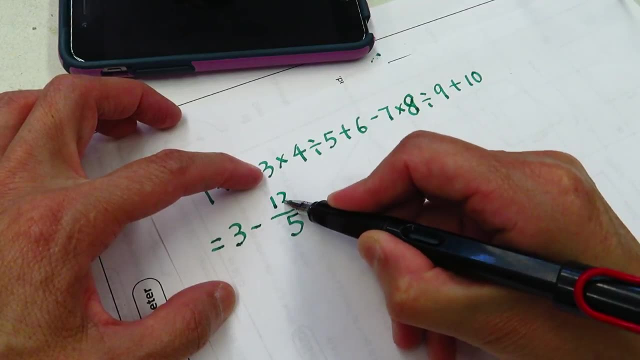 3 minus 3 times 4 times 5.. 3 minus 3 times 4 times 5.. 3 minus 3 times 4 times 5.. Equals 12.. Let's make it 12.. Let's make it 12.. 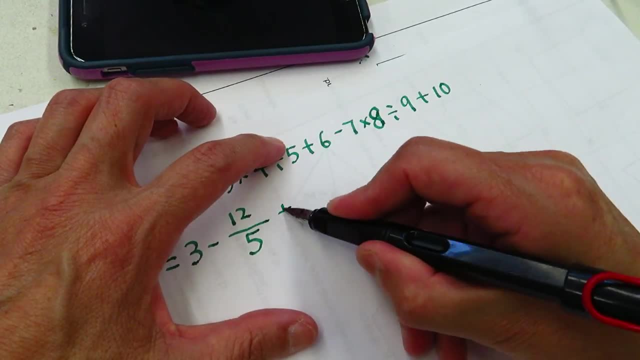 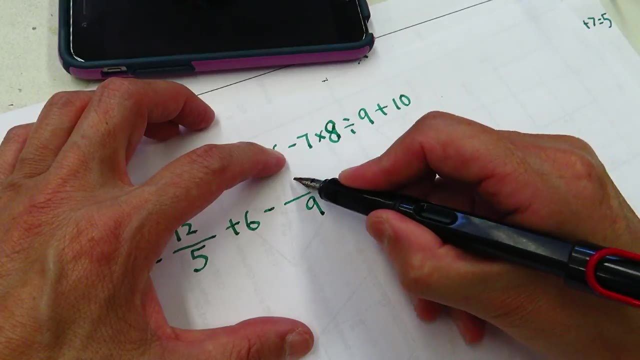 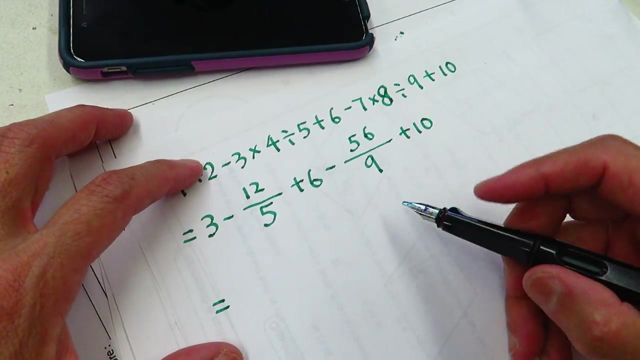 Minus two equals upload. Plus 6 minus 7. Plus 6. 7 times 8 times 9.. Minus 9. 7 times 8. 56 times 10.. Plus 10 plus 10. 3 times 6.. 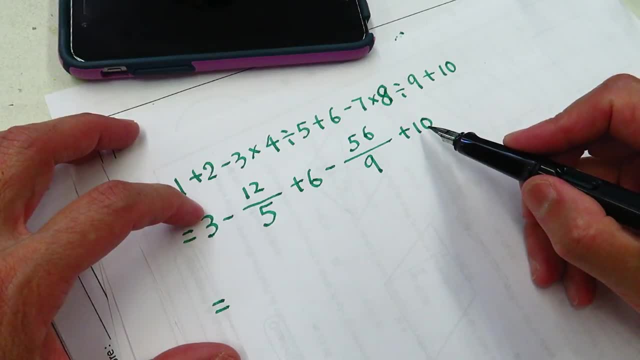 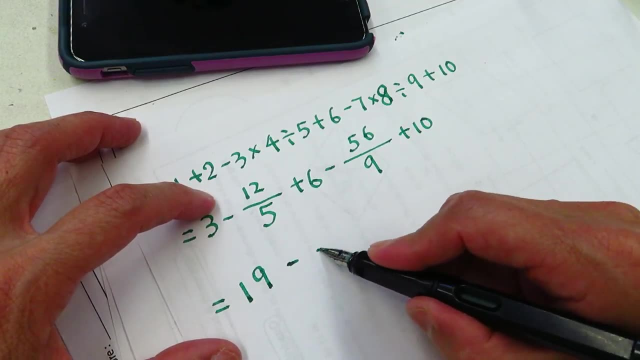 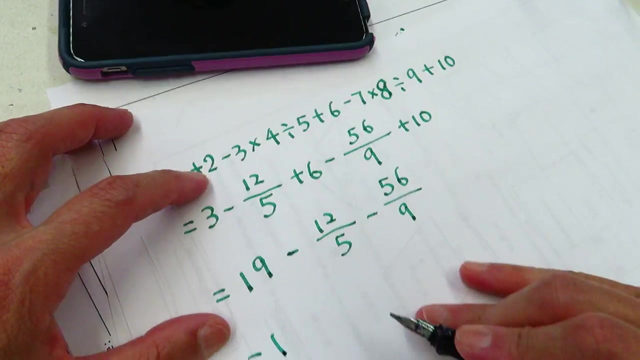 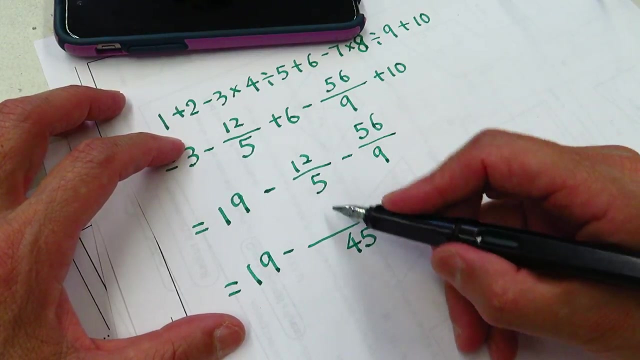 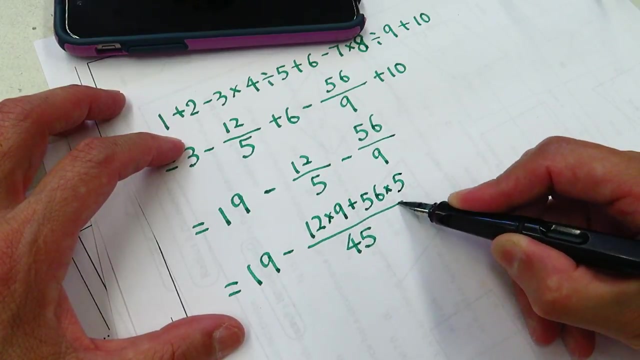 Plus: 10. 19 times 10.. 15 times 19. 19 times 19.. Minus: 5. 10 times 9.. 十二减去九分之五十六等于十九减去五九四十五十二乘以九加五十六乘以五我有点太难了, but the number is not that big, it's ok. 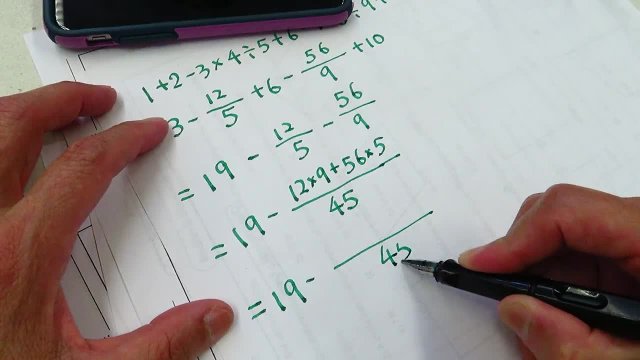 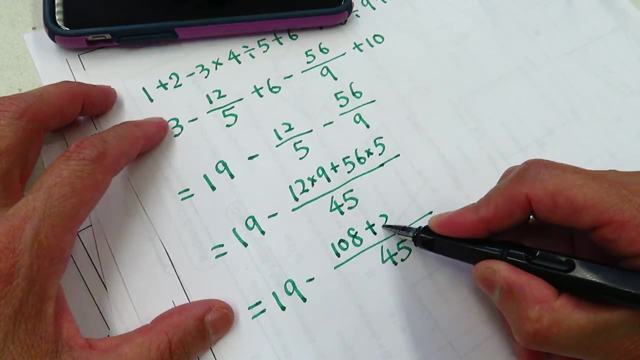 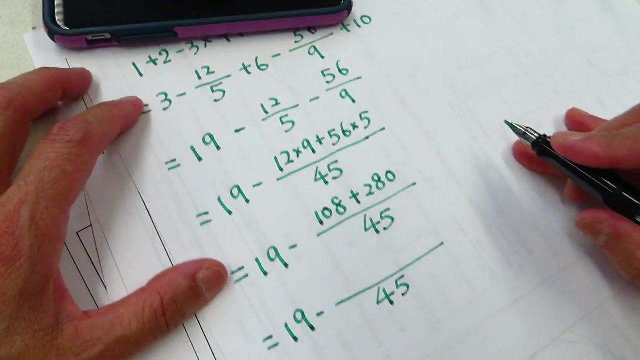 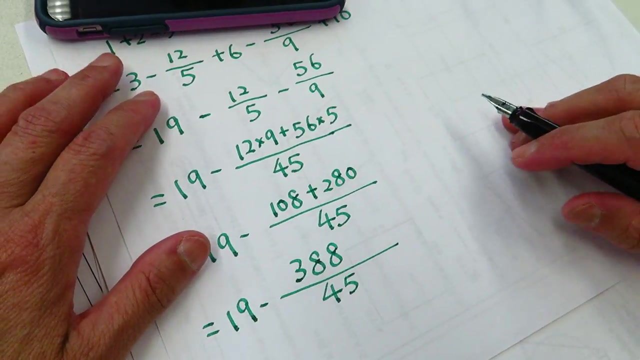 十九减去四十五分之十二乘以九等于一百零八五十六乘以五加上二百八十等于十九减去四十五分之三百八十八三百八十八四十五.